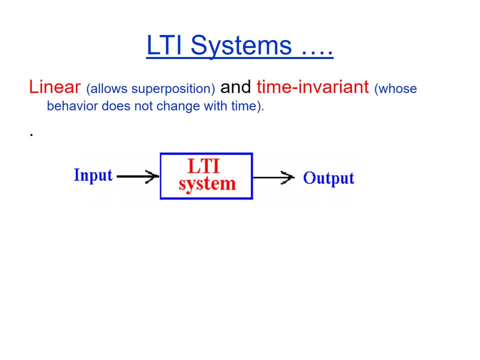 So that is linear. And time invariant means that the behavior of the system does not change with time. So if you work after one or two hours, try to apply a signal after six months, one year. the behavior of the system should remain the same. 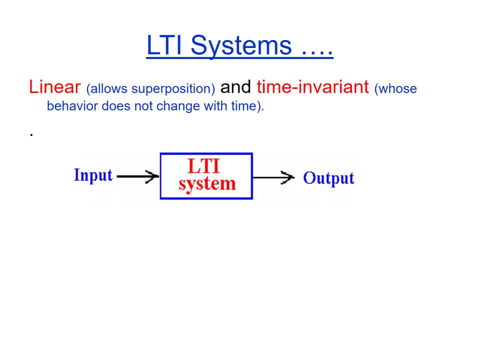 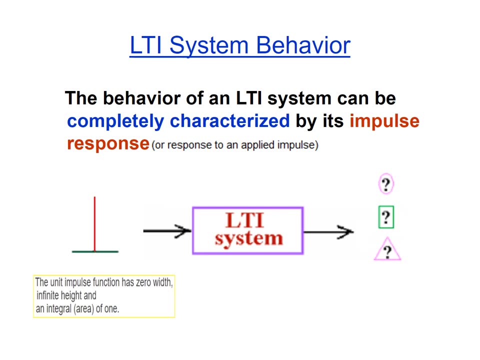 So the combined effect is called the LTI system. Now to judge the behavior of any system, the technique that is followed is that we apply an impulse signal, and the definition of an impulse signal is that it has zero width, So width is virtually zero. 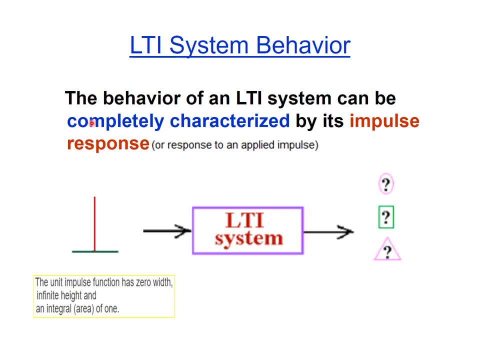 And it has infinite height. So height is virtually infinity And the area is equal to one, So the total area is equal to one. So that is the definition of an impulse input And what we do, that we apply this type of an impulse to the LTI system. 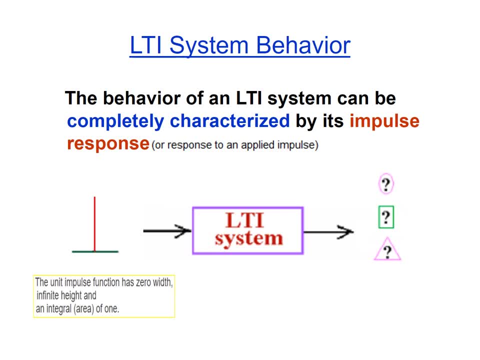 which we want to, whose performance we want to judge. So let's say it's a radio or any other system whose behavior we want to see. So we are applying an impulse signal and we want to see what type of an output we get. 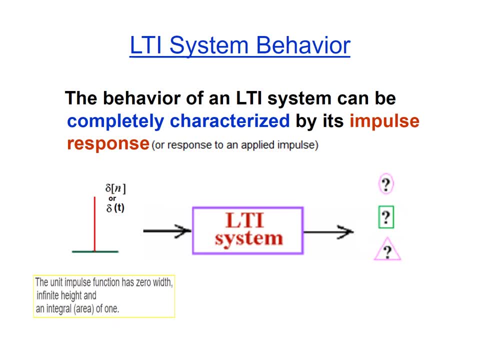 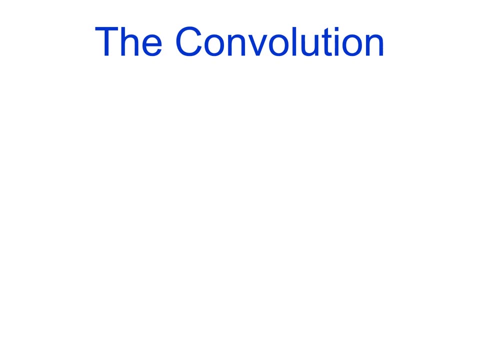 The impulse signal is represented by delta, So delta N for the discrete time signal and delta T for continuous time signal. We'll also be using a term called convolution- Slightly difficult to comprehend, but let's give an effort. So the convolution is a mathematical operation. 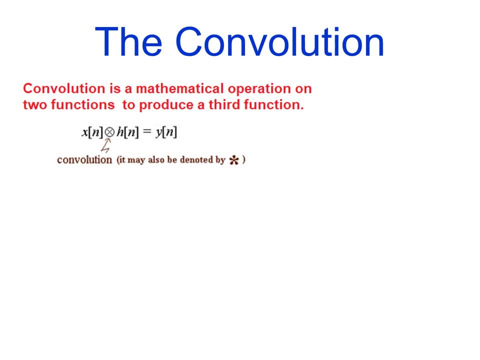 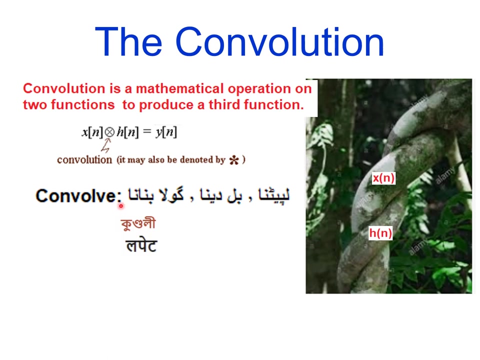 on two functions, two functions- X and H- to produce a third function, YN, And we use this symbol. This is not a multiplication symbol, but this is a convolution symbol. It may also be represented by a simple star. These are the meanings of convolution in Urdu, Bengali and Hindi. 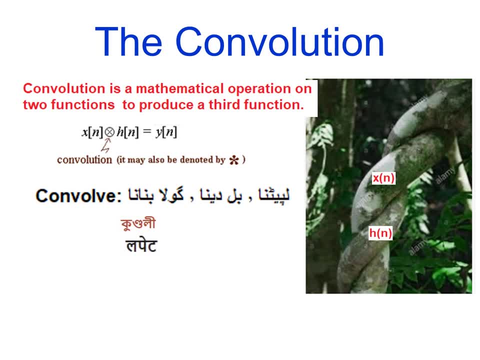 And an idea of what it means really is that if you have two signals- this is the X signal And this is the impulse response- Then the combination of the two is giving the output of the YN signal And formally we define the convolution. 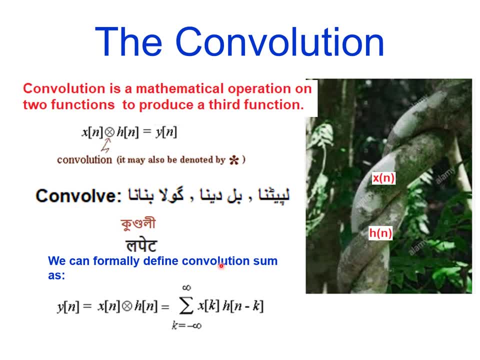 In case of a discrete time signal, we call it convolution sum, And in case of a continuous time signal, we'll call it convolution integral, which we'll see in the next video. So the convolution sum is represented by the summation of the multiplication of the signal and the impulse. 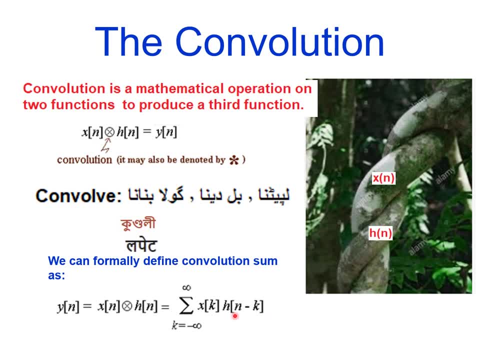 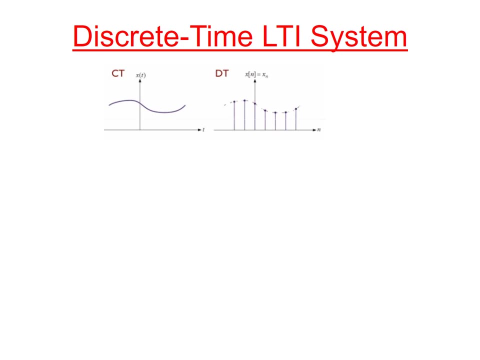 So this is shifted impulse. We'll see what does this mean. And this is integrated. The summation is done from minus infinity to plus infinity. And just to recall, if you remember, this is the continuous time signal And this signal is the discrete time signals. 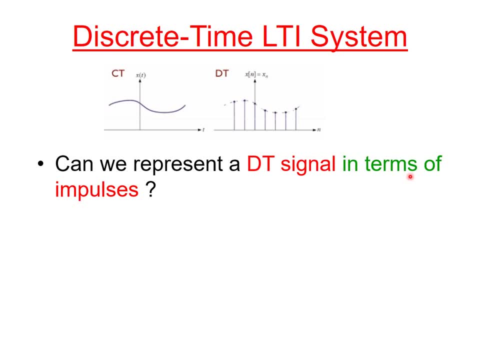 And the question is: can we represent a discrete time signal, the signal in terms of impulses? So, yes, these are impulses, All these are impulses, So we can represent a discrete time signal in terms of impulses. Okay, so this is a signal. 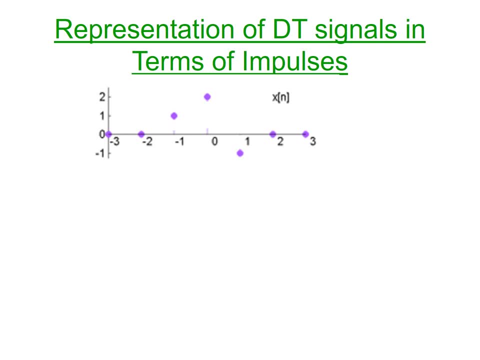 We can see it has a zero value here. zero value here, value one at minus one, value two at zero and value minus one at one. So we can just draw it like this, Draw it like this again. And these are all impulses. 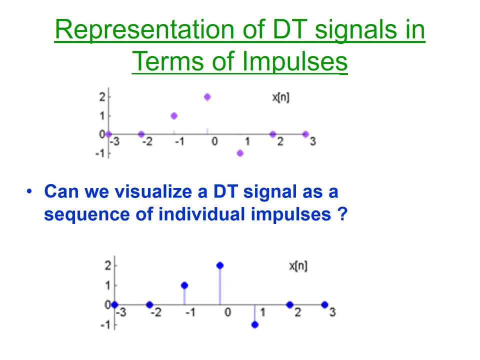 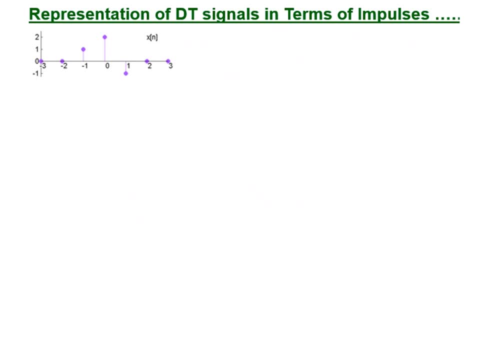 This is one impulse, This is another impulse And this is another impulse. So, okay, so this is the signal And we want to see how it can be represented in terms of impulses. The first signal- here it is at n- is equal to minus one. 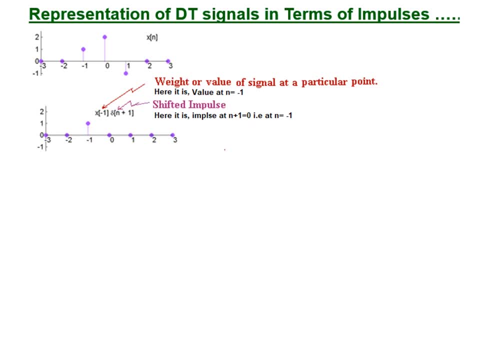 And this is the amplitude. So we write that as x under bracket minus one. This means the weight or value of the signal at that particular point. Here that particular point is n is equal to minus one, So it is written as x minus one. 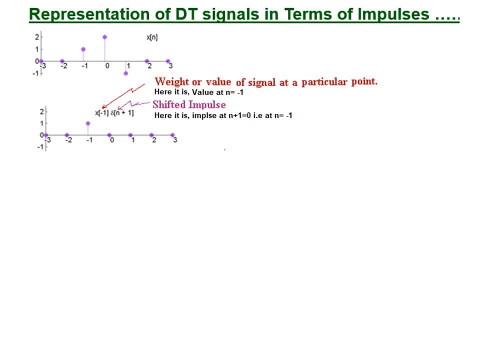 And then it is shifted from zero towards left. So we write it that shifted impulse and delta: n plus one. Why we write n plus one? Because n plus one is equal to zero, means n is equal to minus one. So this is the technique that we follow in naming each of the impulses. 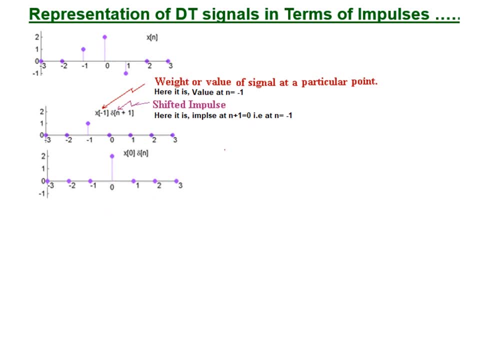 So the second impulse, which is at n, is equal to zero. So we write it x zero because it is at zero And since there is no shifting, so delta is at n And the third one, it is shifted at n, is equal to one. 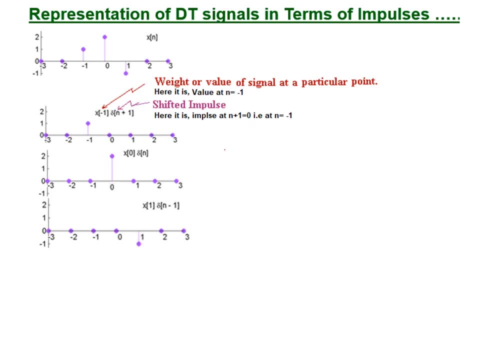 And its amplitude is is given here. So we write it as: x is equal to one And delta is shifted by n minus one. n minus one is equal to zero means n is equal to one. So it is written like this, shown here: 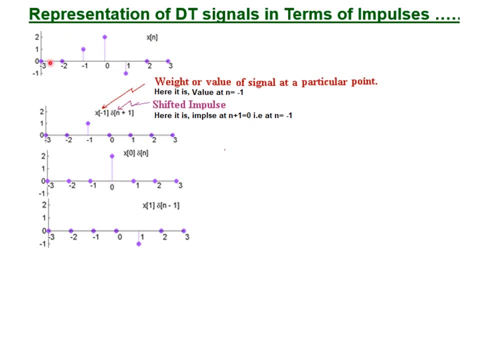 So the signal can be written in terms of a summation of the three impulses. So this is the sum of all three And we can generalize this. We can start from minus infinity to plus infinity. Any signal- not this particular signal, but any signal- can be written as summation of the magnitude and the impulse. 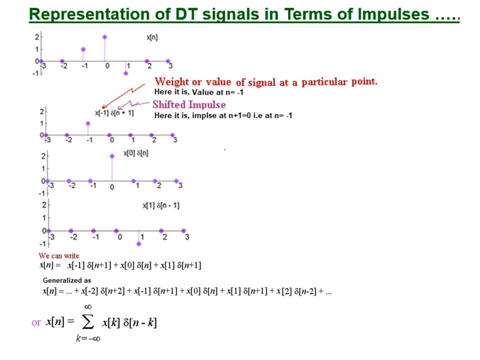 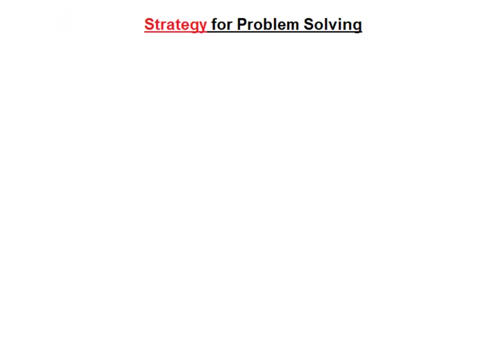 shifted impulse And in a compact form, we can write this signal to be summation of again the magnitude and the shifted impulse. Now, what is the strategy of solving the problems that we? so what we will do here is that we 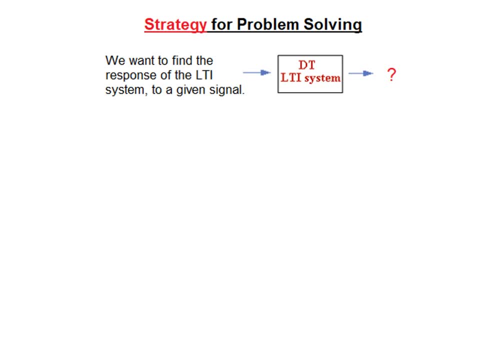 if we have LTI system, we'll try to find the and we want to find the response of the system to a variety of signals. So we apply the signal and we want to know its response. But the first step is to find the impulse response. 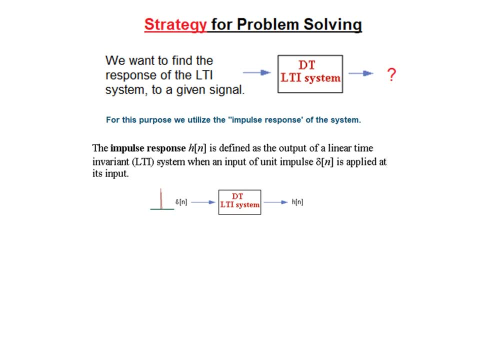 So we apply an impulse to the system and we find its response Hn. And let's say, the response is something like this. So it is funny, but I'll give an example that let's say if the input signal is a barking dog. 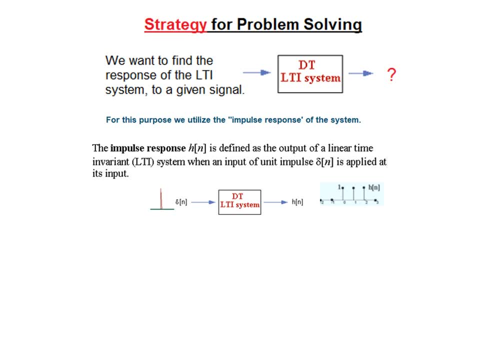 boom. then the output signal we are getting is: wow, wow, wow. So this is the impulse response of this system. Now, if we have an input signal like this, what will be the output? So input signal is like: wow. 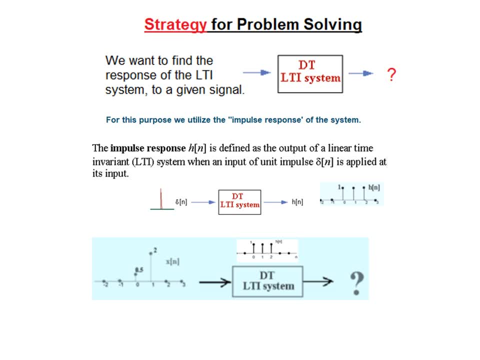 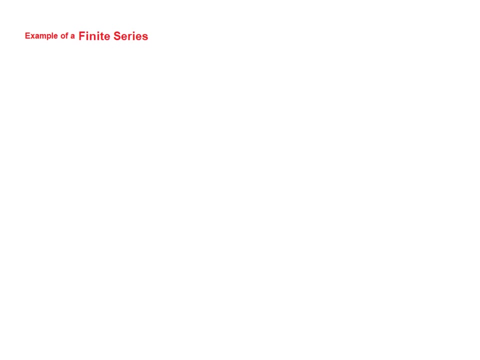 wow, These are the two impulses, And now we want to see what type of an output we will get. Okay, now there could be two types of questions: one involving the finite series, the other involving infinite series. So we'll start with the finite series first. 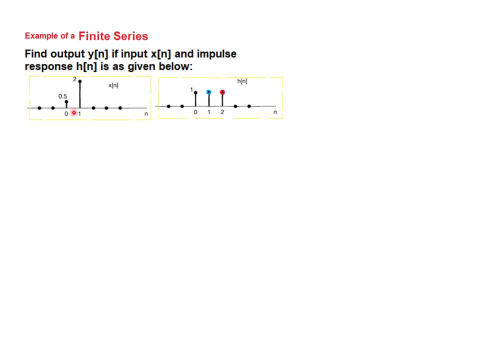 Here is the question. We have an input shown here, Xn, And this is the impulse response of the system. Now we want to find the net output of the system. If you remember, this was the formula of convolution. So output Yn is Xk multiplied by Hnk and summation. 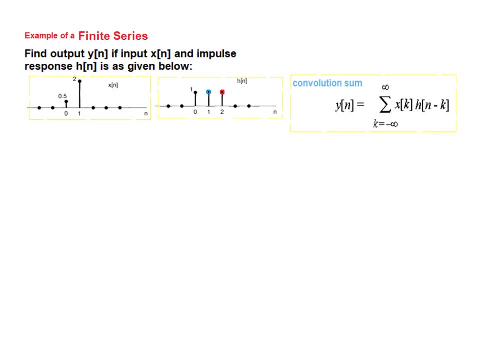 Now keep in mind that this is not delta. this is H. H is the impulse response For convolution sum. we use impulse response. Now the question is: how do we get this term Hn-k Okay? the technique here is that. 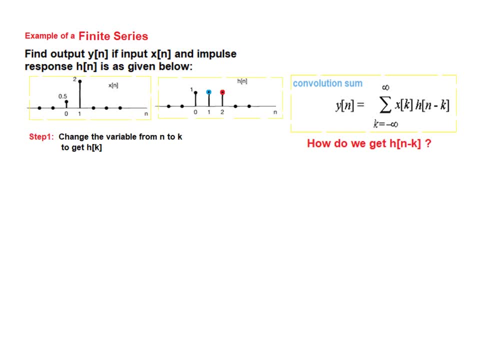 we'll first of all change the variables, both variables n, into k. So this and this, both the variables, have been changed to k, And then we flip this one, the impulse response, along with the zero axis. So zero axis kept intact. 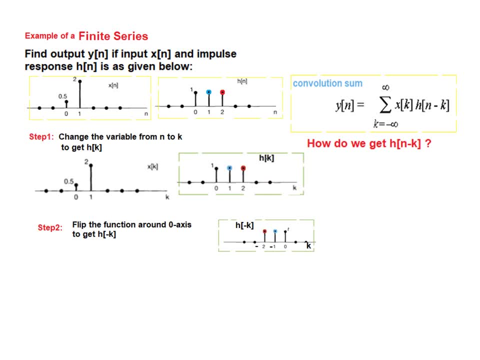 And we flip it on the other side, So it will become like this: So this is now H-k. And then we move it to a point further towards the left, to a point called n, So this signal will now become Hn-k. 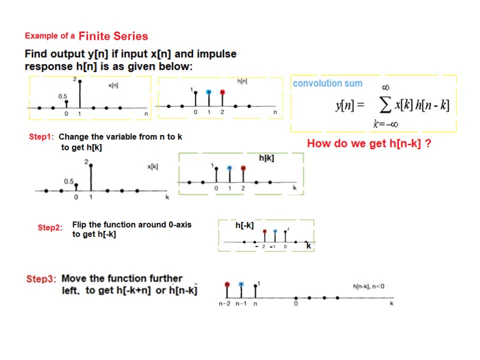 That is, n is shifted to a k, point k. Now, in this case, n is negative, So that is why it will be n-k. Actually, it is minus n minus k, And that will make n is equal to minus 1 or minus 2 or minus 3 or minus 10.. 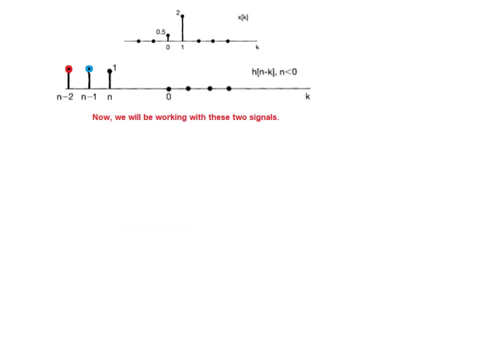 Okay, so we were here And now we will be working with these two signals. So the technique is now that we start pulling this signal- Just assume that it is on a train compartment, mounted on a train compartment. these three signals. Position n. 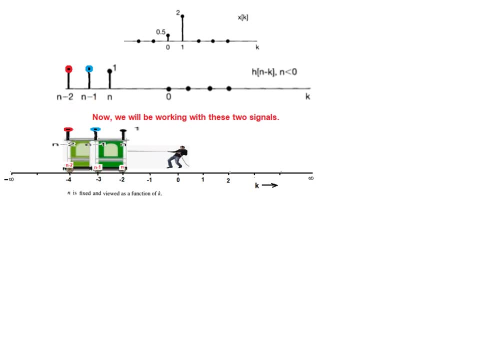 position n minus 1 and position n minus 2.. And the current location is at n is equal to minus 2.. Now we will pull till such time it coincides with the first leftmost signal. Okay, so now you can see that it is coinciding with the first leftmost signal. 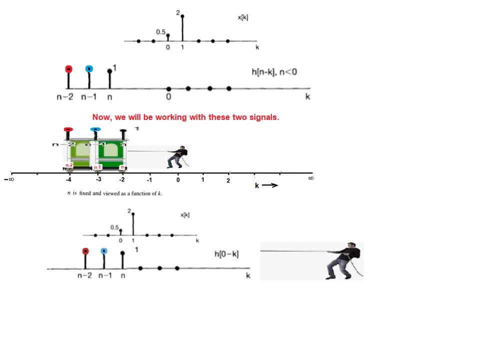 So here we will have an output. Before this there was no output because there was no overlap between the two signals, And so we will call this answer as y0, because now n is at 0. So at, n is equal to 0,. 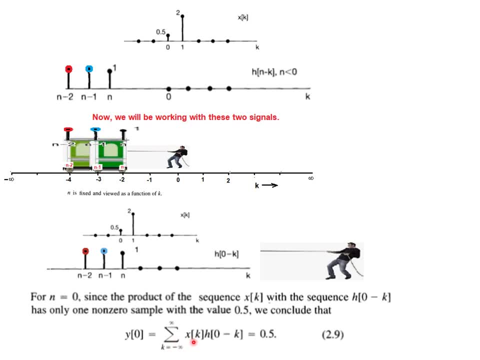 y is 0.. And using the formula xk, h, n minus k, n is 0. So 0 minus k is equal to 0.5.. Now remember the magnitude of h is 1.. 1, all of them. 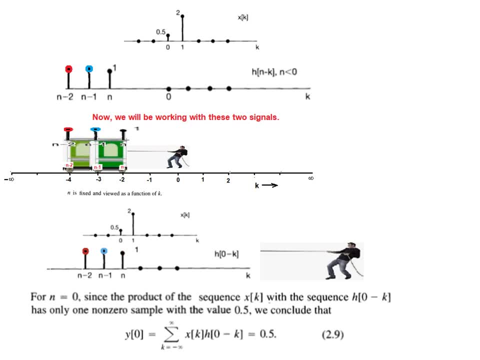 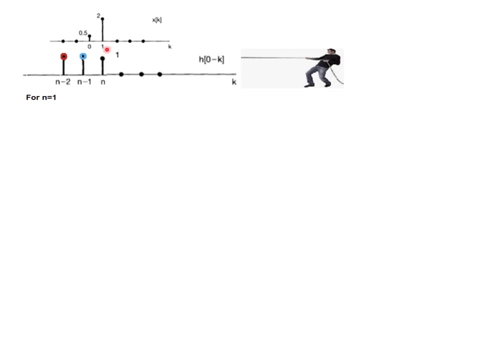 So 1 multiplied by 0.5.. So this is the multiplication of the first overlap. Now let's pull it further to the right. Okay, so when you pull it further now, we have two overlaps, this one and this one. 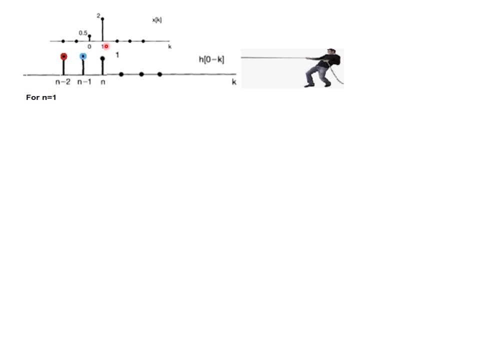 And same way. you can see, now that at n is equal to 1, the sum will be multiplication of this. So 1 multiplied by 0.5 is 0.5.. And 1 multiplied by 2 is 2.. So the total sum will be 2.5. 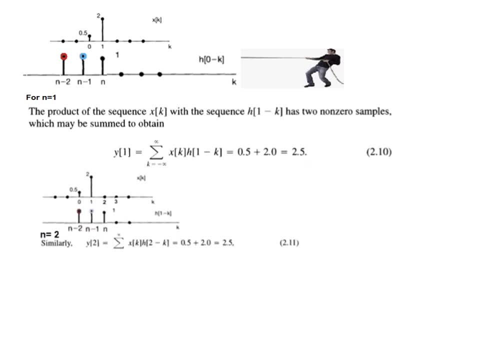 Okay, move it further. So we pull further. This term goes out, So this is overlapping. No, not overlapping, but these two are overlapping. So we'll get a similar result. That is, 1 multiplied by 0.5 is 0.5.. 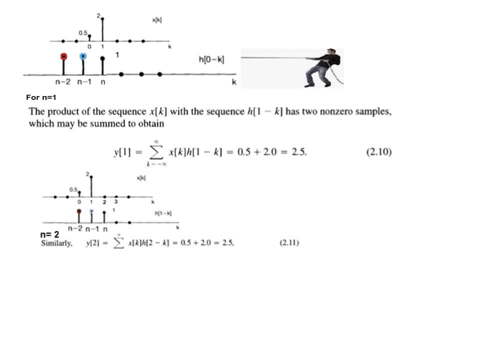 And 1 multiplied by 2 is 2.. So 2.5.. So 2.5 again. Pull it further. Now these two are out. Only 1 is multiplying, And that is 1 multiplied by 2.. So the answer is 2.. 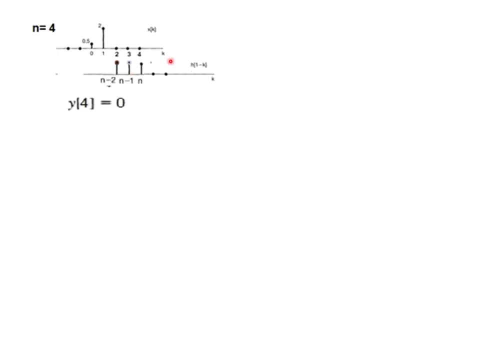 And if you pull it further, there is no more overlap. So the answer in this case will be 0 at n is equal to 4.. n is equal to 4.. No more overlap. Okay, so the net result we can see here. 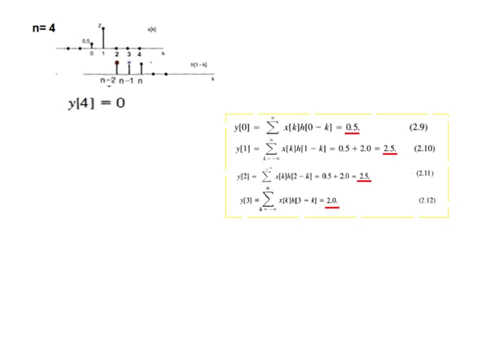 that at y0 it was 0.5,, at y1 it was 2.5, y2 2.5, and y3 2.5.. And so we can plot this signal as shown here. So this is how we solve. 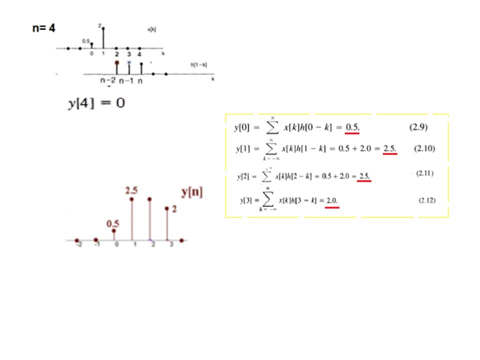 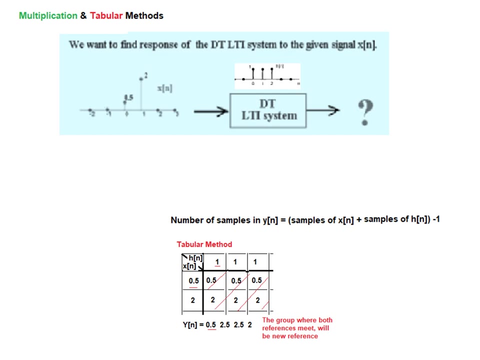 the problems of convolution, And this is basically a graphical technique. We'll have some simple techniques as well, So the same problem- we'll do This- was the input. This is the impulse response And the easiest technique doing by mathematical methods is that we can write it. 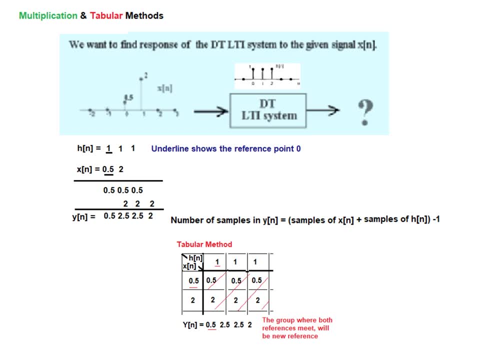 in terms of a number, a figure. So hn is 1, 1, 1.. So we write 1, 1, 1.. And to show the 0 position we put a bar underneath, So underscore: this is showing the reference point. 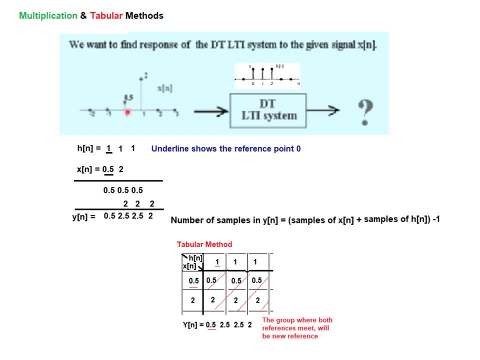 of 0 point. Similarly, for the xn signal, it is 0.5 at the reference point and then 2 at the next two points. Now, the only thing you have to keep in mind that the underlying points or the reference points. 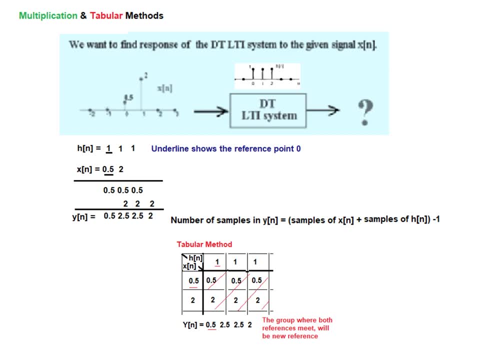 have to be aligned when you are multiplying. So we have aligned these two And now simple multiplication: 0.5 into 1, 0.5, 0.5 into 1, 0.5, 0.5 into 1, 0.5.. 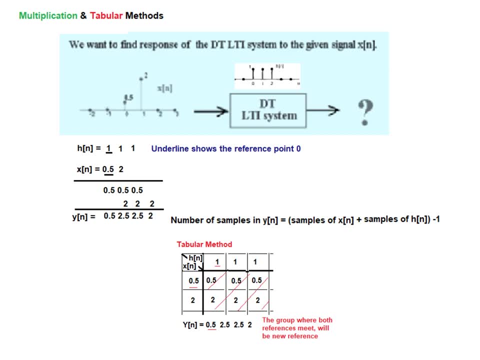 And then the position is the leftmost position you have to write, And then 2,, 2,, 1, 2.. Then again 2 and again 2.. And simple addition will give you the answer that we got. There is another technique. 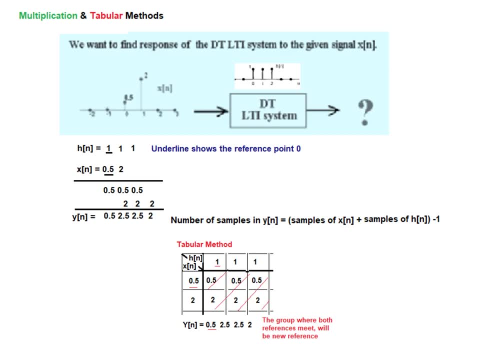 that is the tabular matrix, That is the tabular method. So you create a table hn and xn, hn 1, 1, 1, xn 0.5 and 2.. And then you multiply the 2.. 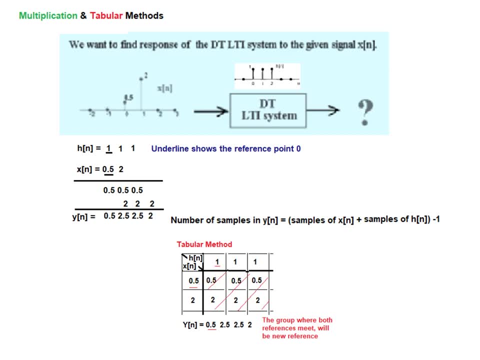 So this is 0.5.. 2 multiplied by 1 is 2.. 2 multiplied by 1 is 2.. So these were all 0.5 and here all 2.. Now you draw the diagonal lines. If you draw diagonal lines, 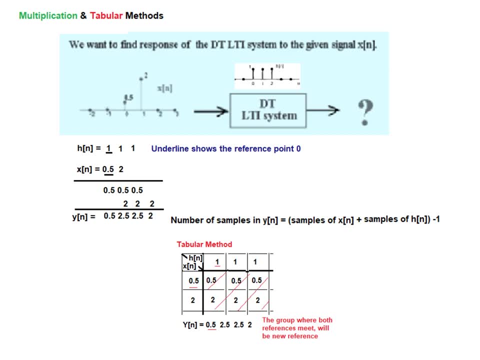 this is for the first point, Or the reference point: 0, 0.. Then the second point is 2 plus 0.5.. So 2.5.. The third point is 2 plus 0.5.. 2.5.. 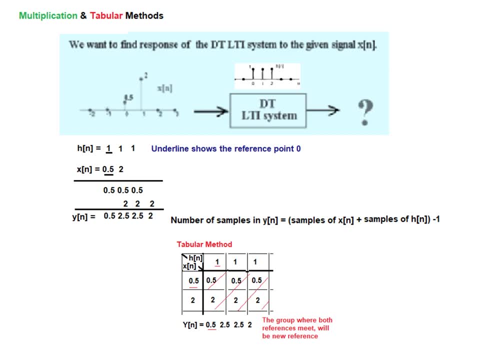 And the fourth point is 2. So you get the same result that we got here or that we got in the previous way, But this, I don't think, gives you a real sense of what is done. So it is better to understand the graphical method. 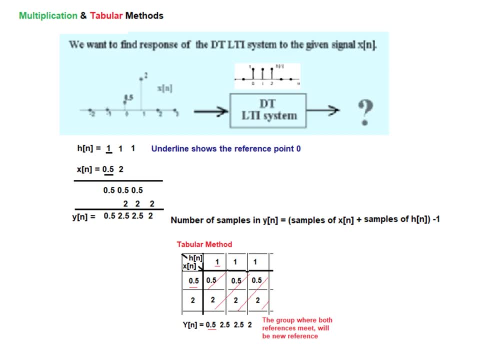 And this can be used for checking your answer. And in the final answer also, you have to keep in mind the align, the reference points. That is important And wherever the reference point, the answer reference point, should also be there And you can plot. 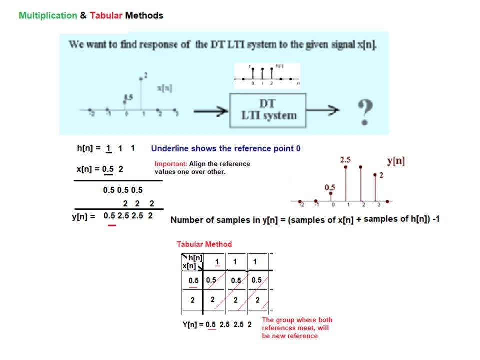 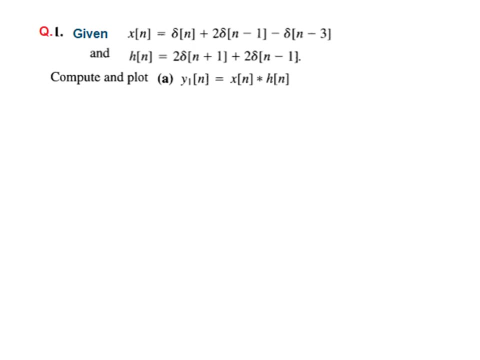 and it is the same plot that we got through the graphical method. Here is another example: Two signals, Xn and Hn, are written in terms of their magnitude and the shift Impulse shift And we need to find out the convolution sum. 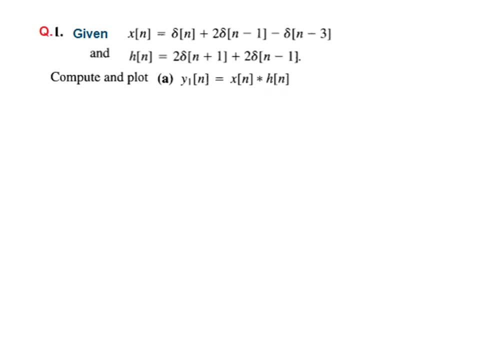 or output Yn. So let's first of all draw the two signals. From here you can see that this is at no shift and shift 0, that is at point 0. its magnitude is 1.. Multiply by 1, so we write it at point 0. 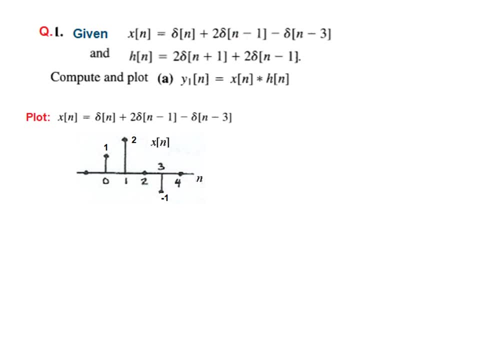 magnitude is 1.. Then at n minus 1, that is at n minus 1 equals 0. that means at n is equal to plus 1. So at n is equal to plus 1, the magnitude is 2. So we draw a line of length 2.. 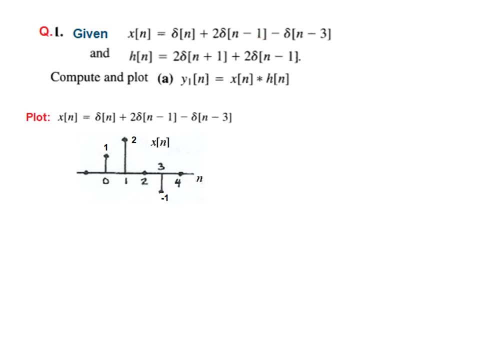 Then there is no n minus 2. that means at n is equal to 2, the magnitude is 0. So we plot it like this: And then n minus 3 have a magnitude of minus 1. So at 3 the magnitude is minus 1.. 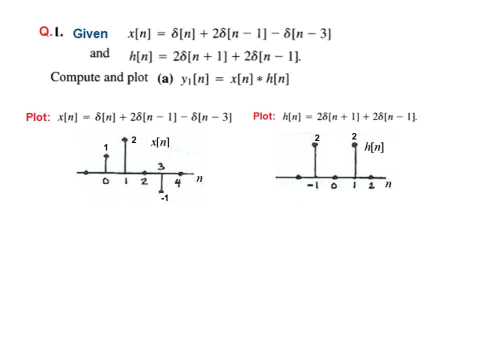 Similarly we plot Hn Two: amplitude at shifted point minus 1. So at minus 1 it is 2.. And 2 amplitude at shifted point plus 1.. So at plus 1 it is 2.. And at 0 point: 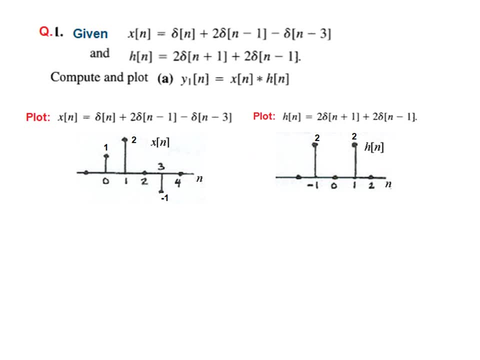 there is no signal, that means it is 0.. So these are the two signals in graphical forms And, as I mentioned earlier, it is better that you learn the technique of graphical convolution, But here we will take the shortcut method, that is, the mathematical method. 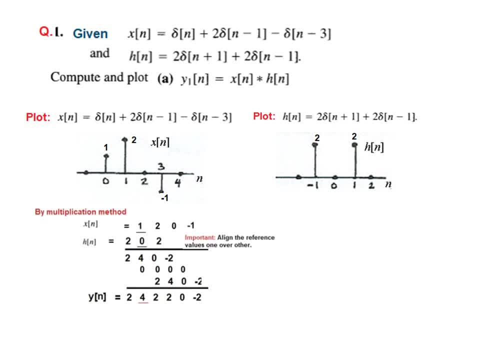 or the multiplication method. Okay, So these two signals: Xn. 1, 2 0 minus 1, 1, 2 0 minus 1, the amplitude of the signals we have written- And similarly Hn is 2 0, 2. 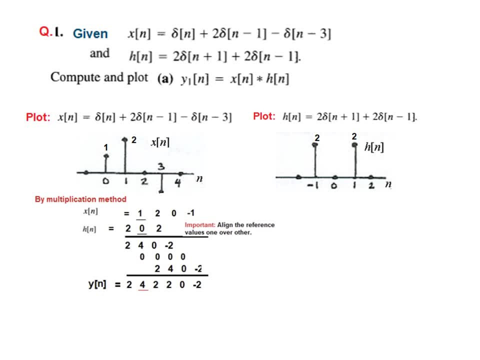 So 2 0, 2, We have to align the reference values. that is important. So before multiplication you must align the reference points And then you start multiplying and you start writing from the leftmost point. So this is the leftmost point. 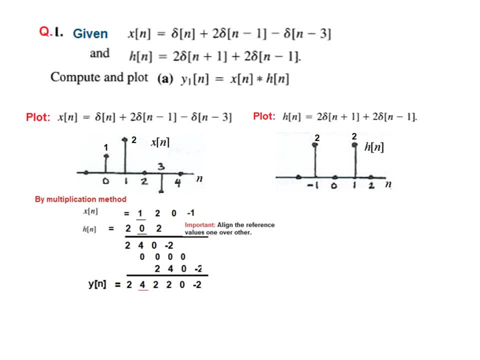 So 2 1, 0, 2 and 2 2 0, 4. so simple multiplication, Then another line and then the third line And then simple addition. So 2 4, 2, and this is 4 minus 2 is 2.. 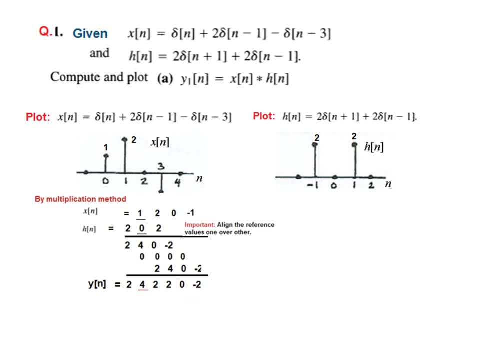 0 and minus 2.. So this is the answer. Now the same operation can be done by: if you write Hn at the top and Xn at the bottom, No problem, Just keep in mind to align the reference points And you start writing from the leftmost point. 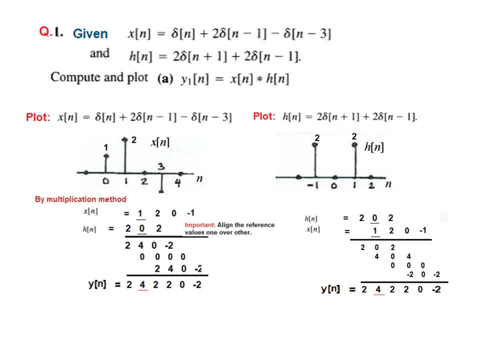 So 1 2 0, 2. So we write here, not here, 1 2 0, 2, leftmost point, And then all the 4 steps And then multiplication, So you get the same answer. So we can write it. 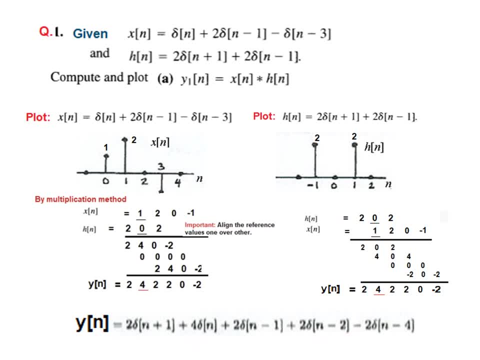 in terms of delta. now That Yn is 2 delta n plus 1. This was the 0 point That is shifted left, Then at 0 it is 4.. So 4 delta n- Keep on moving. 2 delta n minus 1.. 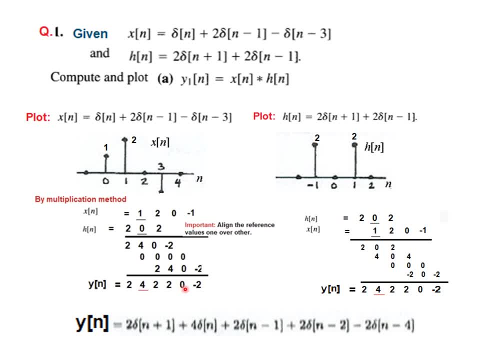 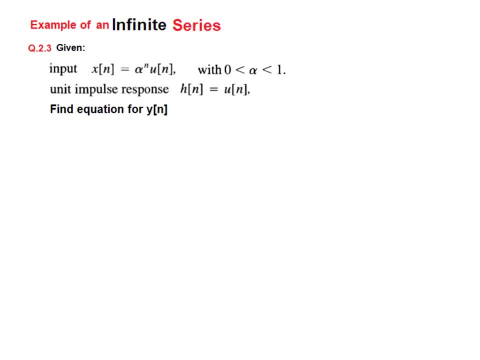 2 delta n minus 2.. And 3 is 0. So we don't write Then: minus 2 delta n minus 4.. So this is the final answer. Okay, our next example is of an infinite series. We did last two examples. 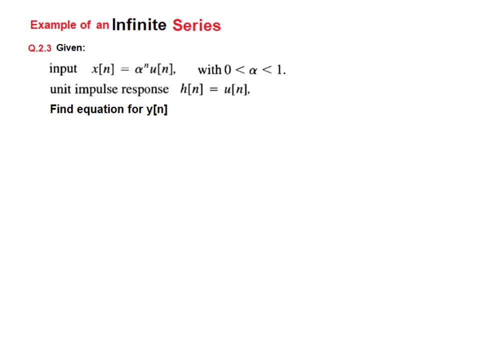 of a finite series. So let's see, This is the input signal. Xn is alpha power, n, Un, And I hope you know what is the meaning of Un. That is, it is towards the right hand side of 0.. The signal is present. 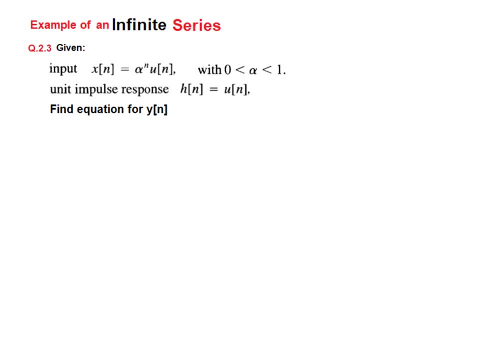 towards the right hand side of 0. Nothing on the left. And also alpha is defined to be have a value between 0 and 1. And the unit impulse Hn is Un, So it is also impulses on the right hand side. 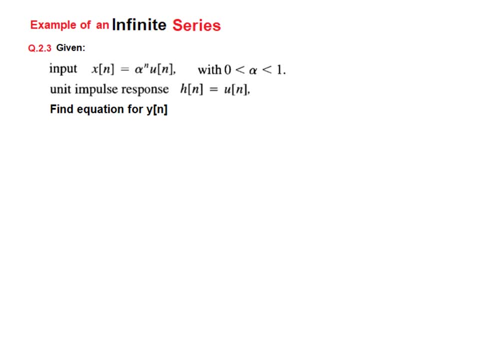 And we have to find the equation for the output Yn. So for our ease we just assume a value of alpha. Let's say it is 0.9.. So alpha power n or alpha power 1 will be 0.9.. 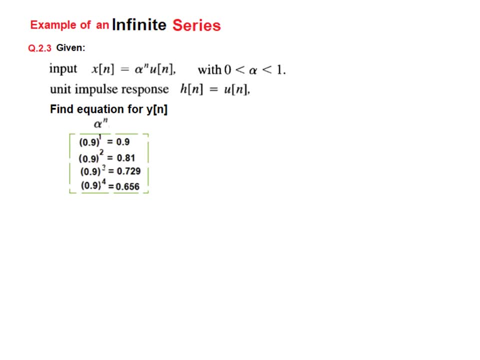 Alpha power 2 will be 0.81.. Alpha power 3: 0.729.. Alpha power 4 is 0.659.. So this will give us an idea as to the shape of the plot. Okay, So now you can see from here. 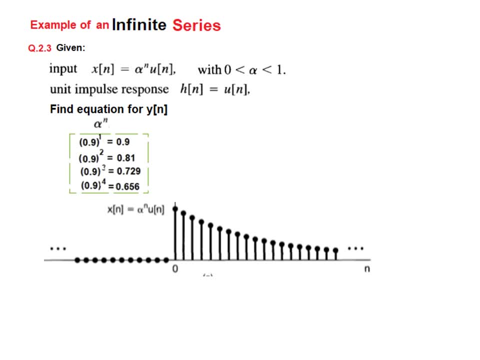 that it is gradually decreasing: 0.9, then 0.8, then 0.7, 0.6. So we'll draw it like this. So this is the shape of the input And it is since, because of the Un, the signal is only present. 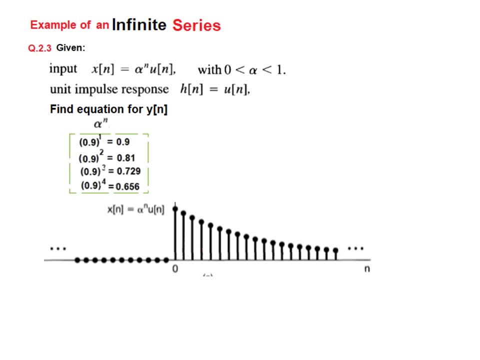 on the right hand side of 0.. And Un we recall from our earlier knowledge that unit step function in time domain is like this And it is in a discrete time. it will be like shown here. So the amplitude is 1 and it is only on the right hand side of 0. 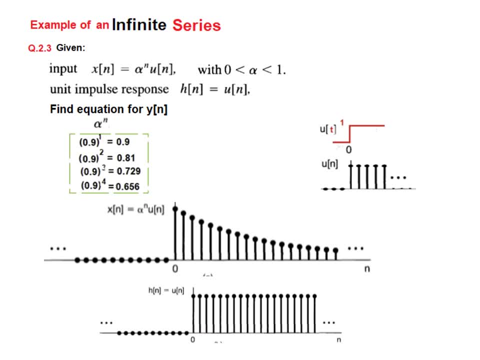 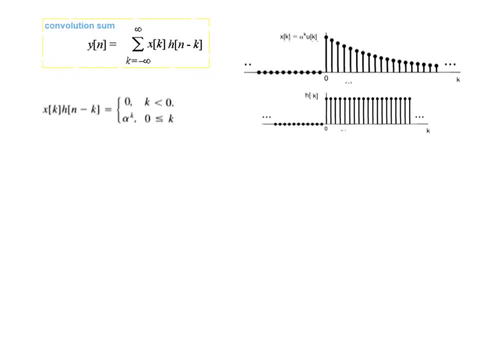 So in this case also, our Hn will be something like this: and it is going to infinity, This is also going to infinity, This is also going to infinity. That is why we call it a infinite series. Okay, Now, it is very difficult to. 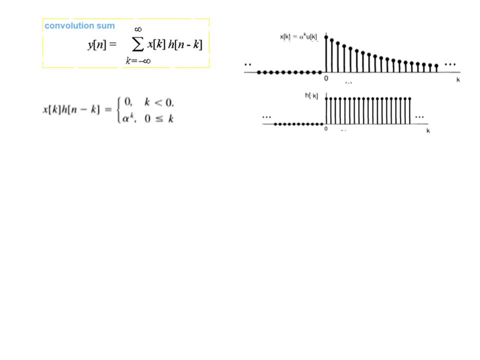 do it graphically by following each step or pulling each step, But we have to keep in mind the same technique. Okay, Now let's first of all find the multiplication part. The multiplication of the two terms will be 0 for k less than 0.. 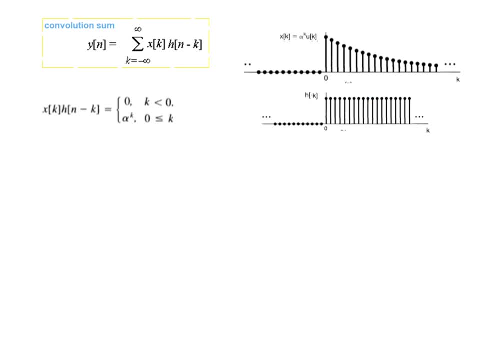 We have converted the scale to k, as in the last two examples. also From n. we have converted this to scale k. So for k less than 0 the output will be or the multiplication will be 0. But for k greater than 0, 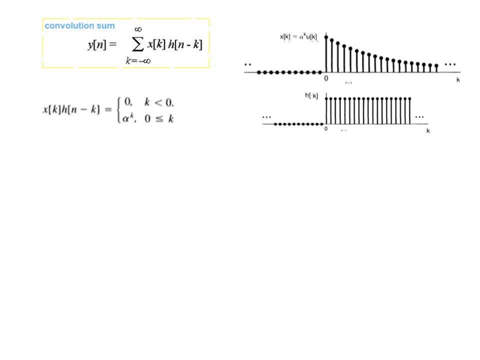 since this is 1, so 1 multiplied by ak will be ak, So it is ak. So this is how we get the general term of the multiplications And now the summation term. So in this equation, now this term, we have found out. 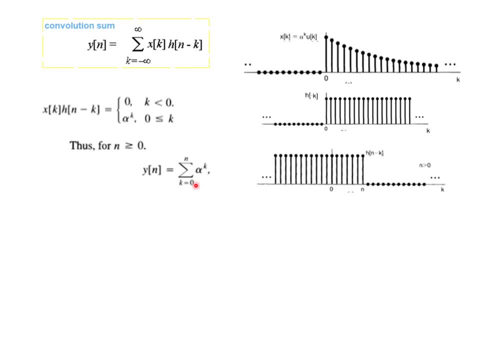 to be ak for k0 to n or on the positive hand side. So now the output will be: the output can be written as: from k0 to n, a less to the power k, This one. And now we will take help of a geometric formula. 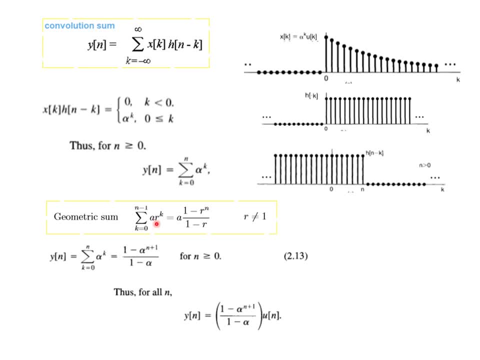 So this is a geometric formula that the summation of a rk is given by a, 1 minus rn, divided by 1 minus r. Now if we compare with our case, then here a is 1 and for r we have alpha and k remains k. 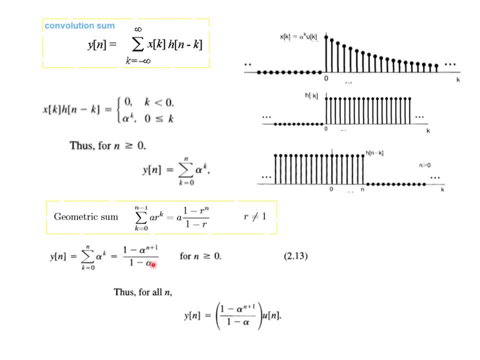 So we replace the rs with alpha. So this is the equation in our case. So we can write it that for all n we just multiply it by un. This is the output equation: yn is 1 minus alpha, n power 1. divided by 1 minus alpha. 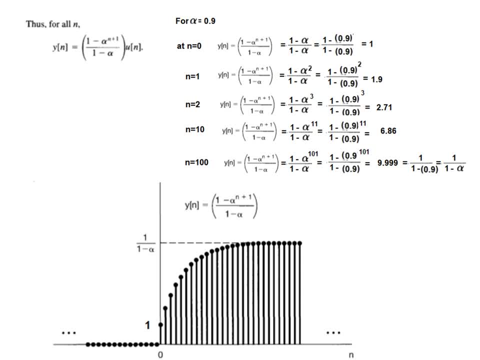 Ok, Now to get an idea about how the plot will look like. This was the output and we just take couple of values: of n And we had. alpha is equal to 0.9. that we had assumed. So when n is 0, 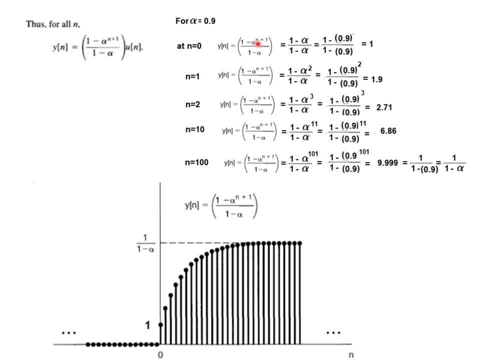 this term will become 1 minus alpha, So 1 minus alpha at the top and 1 minus alpha at the bottom. So this will become 1. if you want, You can just put the value of alpha 0.99. still the answer remains 1..